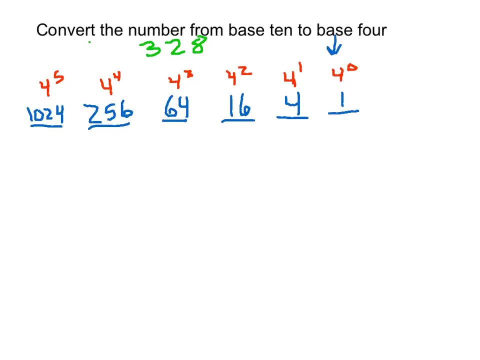 4,096, something like that- How do I know? not to continue. Well, what you want to do is go to continue to do powers of 4, or powers of 3, powers of whatever base you're converting to. 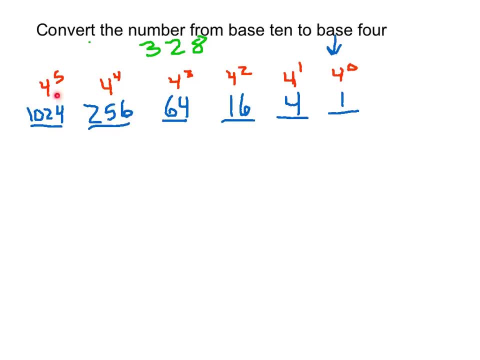 until you get to the number the first time that that particular place value is larger than the number you're given. So we're given 328.. We can continue to go until we get to a number larger than 328, and then we can stop. 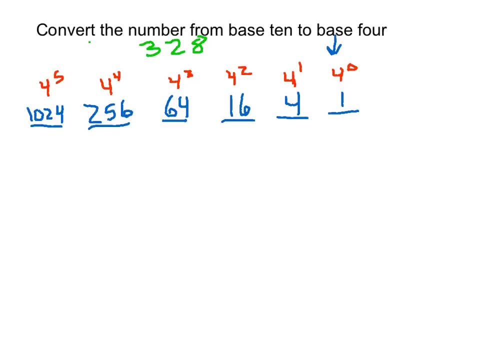 Now we're going to be in base 4.. So when you're in base 4, you know that you're only allowed to use the digits 0,, 1,, 2, and 3.. We're only allowed to use the digits 0,, 1,, 2, and 3.. 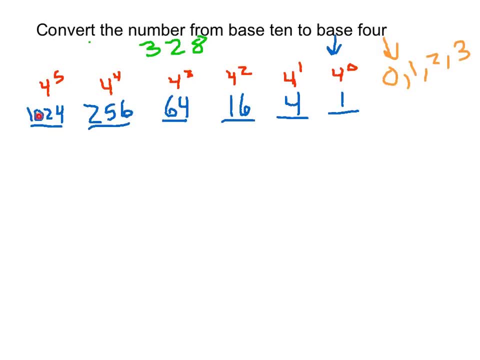 And we need to place them in these particular values here. these place values, these columns, in order to represent 328 objects. So if we were to put- and this is going to be a little bit more complicated- but if we were to put- and this is going to be a little bit more complicated- 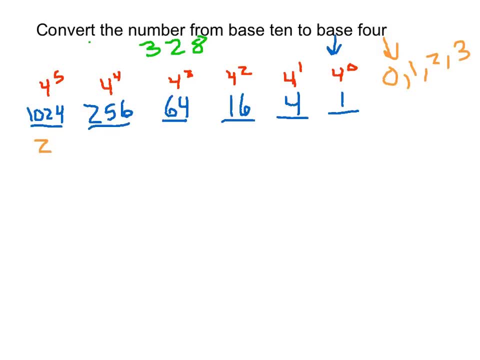 but if I were to put a 2 in this particular column, what this represents? a 2 in this column represents 2 times 1024.. And we know that this is going to be a certain amount of objects much larger than 328.. 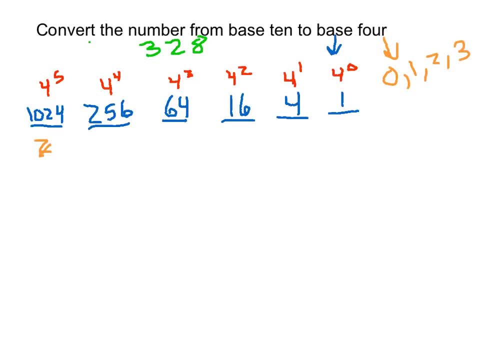 In fact, if I put any number in there, if I put any number in there, this is wrong. If I put any number in there other than 0, it's going to be larger than 328.. So I know that. no digit. 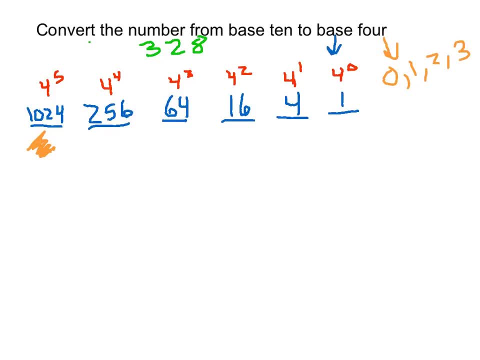 It's going to go into this 1024 column. We do see that 256, there are 256 objects that go into 328.. The question is: how many, How many? how many times does 256 go into 328?? We see that, really, it only goes in one time, right. 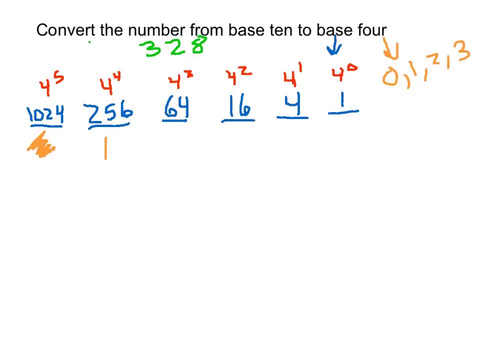 One group of 256 goes into 328. So putting a 1 in this column gives us 256 objects. now we need to fill in these other columns. So what we want to see is: okay, this represents 256, how many of the 328 we originally had are left over? 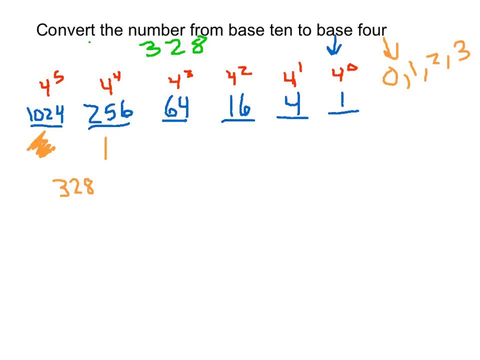 So we have 328, and we, just by putting that 1 in that column, we just represented 256.. So how many are we going to have? This is going to be 2, this is going to be 7.. We're going to have 72 objects. 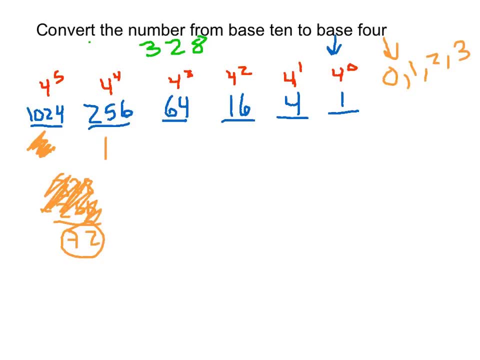 So just by putting a 1 in this column, we want to know how can we use the digits 0,, 1,, 2, and 3 and place them strategically in these columns to represent 72.. Notice, I don't want to put another. I don't want to increase this to 2, because if I put 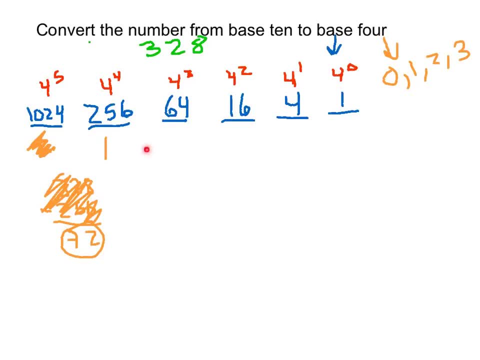 2, that would be larger than 72. So how many times does 64 go into 72?? Obviously We want to see that that's just 1.. If we put any other digit other than 1,, if we put 2 or 3,, then we see that this particular 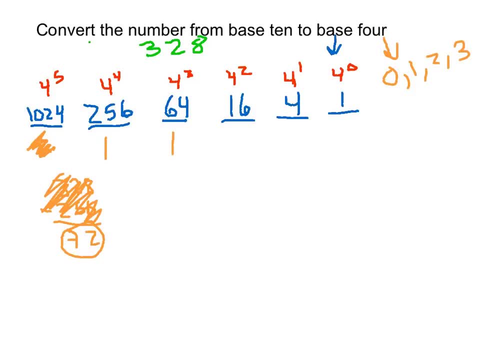 number would be larger than 72. So only one group of 64 goes into 72. So, putting that 64 there, what's left? Well, this will be 8, and this will cancel out. So now we need to represent 8 objects using these columns. 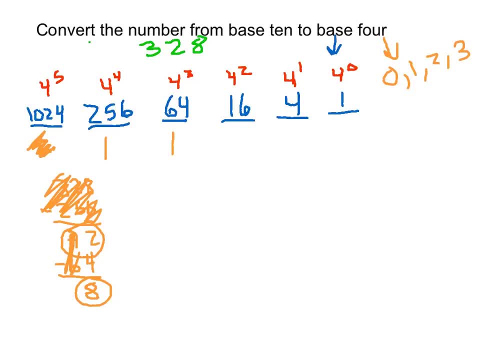 So we need to put 0s, 1s, 2s and 3s in these columns here, where every number that goes in this particular column represents a group of 16.. Every digit that goes in here represents a group of 4 and groups of 1.. 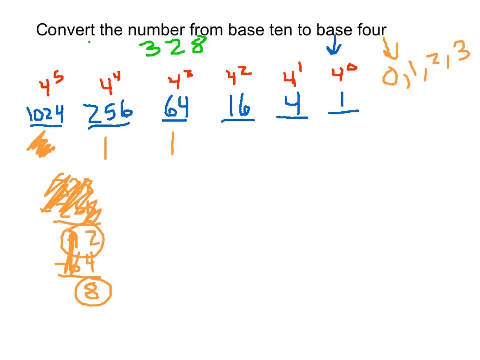 So how many times does 16 go into 8?? Well, 16 does not go into 8.. So there are going to be 0 groups of 16 that we can make with 8 objects. How many times does 4 go into 8?? Well, 8 divided by 4 gives us 2.. So if we were to subtract that, we would have 0 left over, which means we have 0- 1s. So this would be our number: 11020.. This would be our number in base 4.. 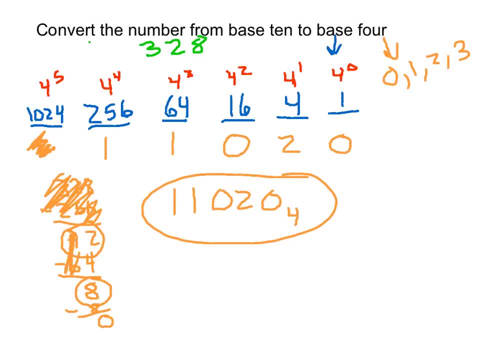 If we wanted to talk about 328 objects, that's the same as talking about the number 11020 in base 4.. Because each particular value right, Each place value, Each column represents a different power of 4.. So this would be the 1s place, the 4s place, the 16,, the 64,, the 256. 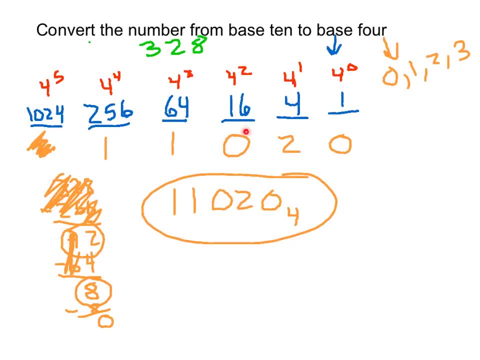 And what we want to do is to first figure out the value of each column and then think about how we can place the digits 0,, 1,, 2, and 3 in those columns to represent the number 328.. Let's look at another example. 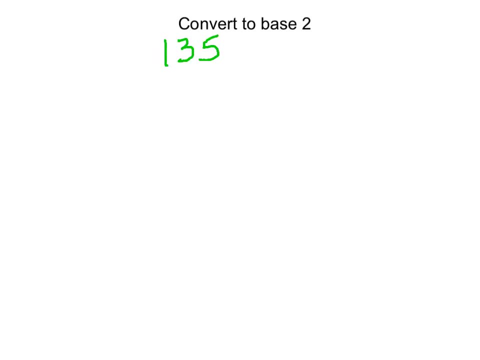 Okay, Let's do another example. We're going to convert this number to base 2.. We are given a number- 135, and I know now that we have discussed what different bases mean. you might be saying: how do I know that's not in a different base? 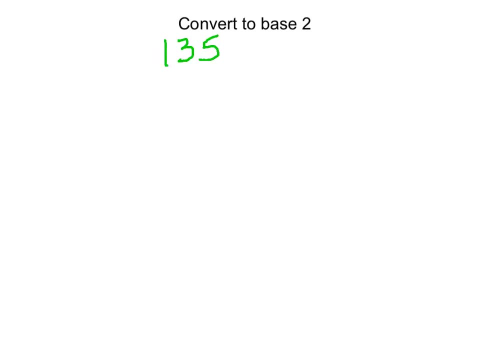 Well, if we don't see a little sub-number here, then we assume it's base 10.. So we're in base 10.. This represents 1 group of 100,, 3 groups of 10,, 5 groups of 1, and we want to convert. 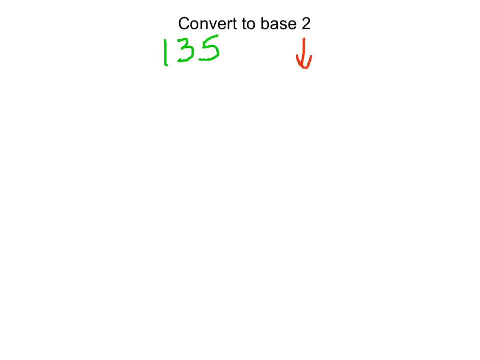 this to base 2.. As soon as I see that it's base 2, I'm going to start by labeling. I'm going to start by labeling each column. So we have the. we always have the ones column. right, We have the ones column. 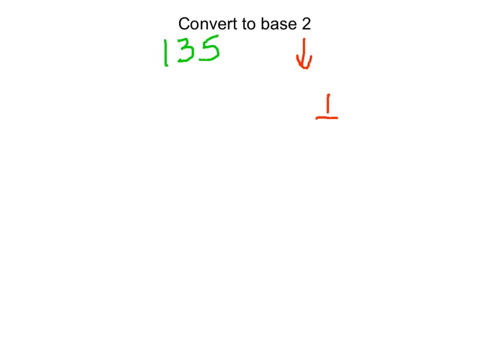 And then now we're going to go up by powers of 2, so we're going to continually multiply by 2.. We have ones. Multiply that by 2, we have this twos column. Multiply that by 2, we have the fours, the eights, the 16,, the 32s, the 64, and the 128.. 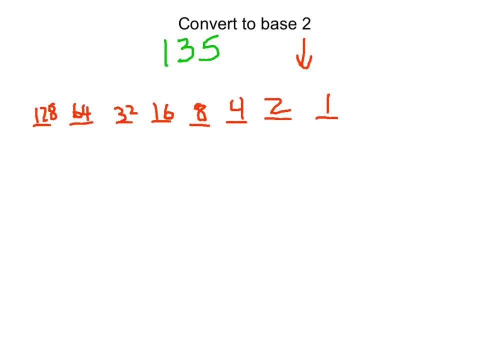 Now I'm going to stop there. Okay, I'm going to stop there, not only because I'm out of room, but because you can see, if I were to multiply by 2 again, I would get a number that's larger than 135.. 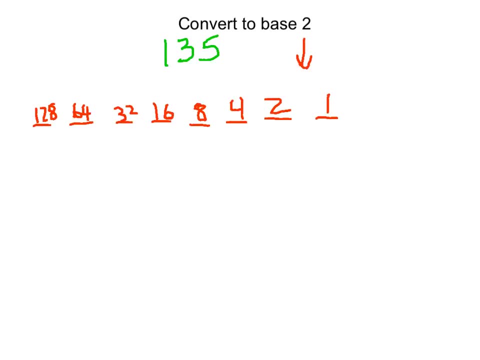 So these are the only columns that I need. We want to get up to the column that's- you know, the column that is the one that's one less than the larger number. So if we were to multiply this again, we get 256. 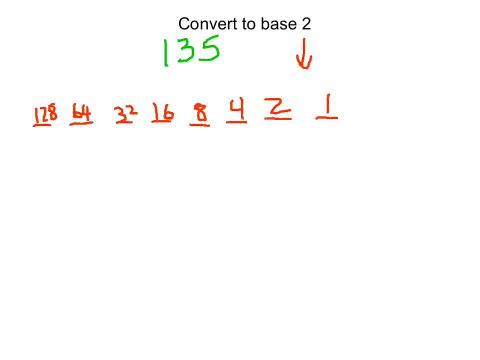 That's larger than 135, so we can erase that column. Now we're in base 2.. So what numbers are we allowed to use in base 2? What numerals, What symbols are we allowed to use? Well, we're always allowed to use zeros and we're always allowed to use ones. 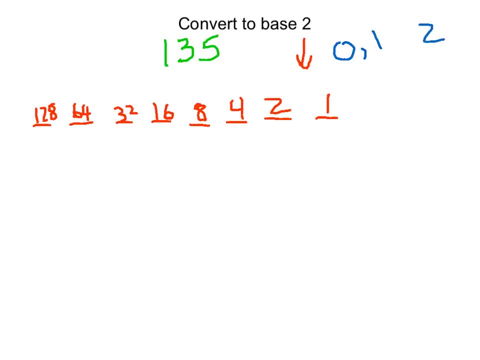 But in base 2, we're not allowed to use the symbol for 2.. That symbol for 2 does not exist in base 2.. We can represent it in base 2, but we do not include the number in that particular. that. 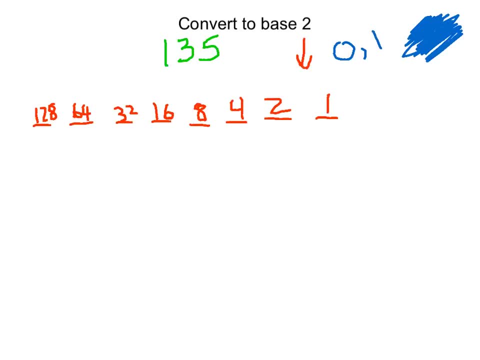 symbol in that base. So what we want to do is strategically put zeros and ones in these columns in order to get a number that equals 135.. So if you think about that, how many times let's start? we always should start the furthest. 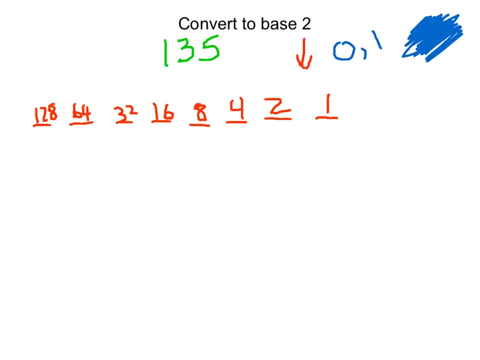 to the left column, right, The largest column that we can start in. So how many times does 128 go into 135?? Okay, Well, we have two choices: It goes in zero times or it goes in one time. And we know it's not zero because 135 is larger than 128, which means, if you were to have 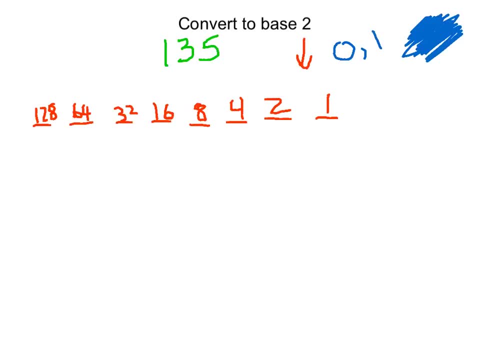 135 objects spread out, you could find 128 of them. So we have one group. let me change colors here. we have one group of 128 that goes into 135.. So just by grouping- If we started with 135, and just by putting that one there that represents 128. 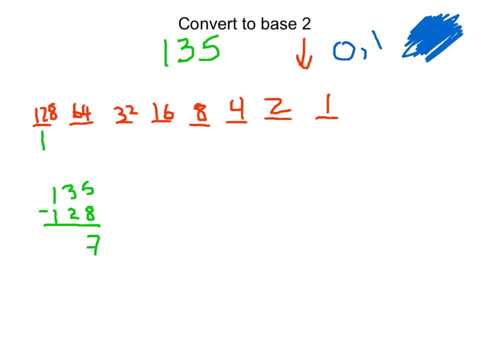 So how many are left over? Well, it looks like we only have seven Right. So just by putting this one in this column, we now need to put zeros and ones in the remaining columns in order to represent the number seven. So we see that. how many times does 64 go? 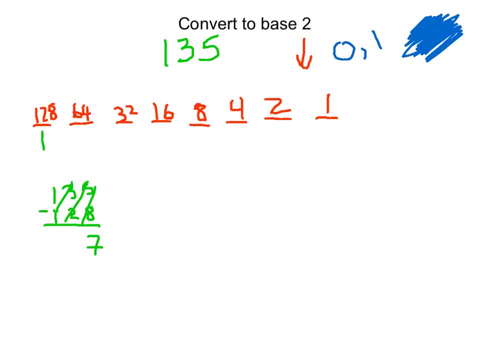 It goes in zero times. So how many times does 64 go into seven? We have seven objects. We need to be able to group 64 of them together. Well, that's going to happen zero times. We're not going to be able to have that happen. 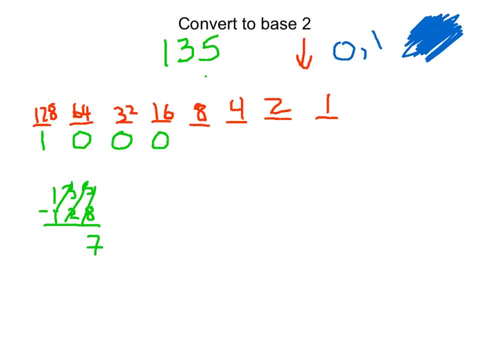 Same thing with 32.. Same thing with 16.. Again, same thing with eight. So we're going to put zeros in all these columns, because if we were to put the number one in any of these columns, we would be larger than seven. 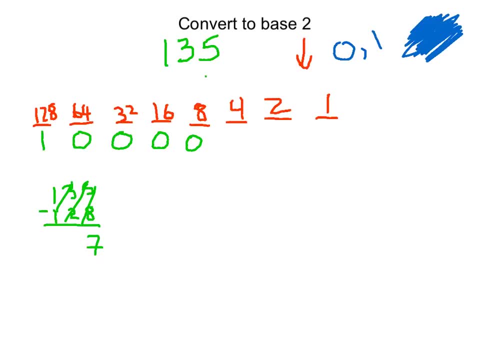 We only have seven left over. So how many times does four? We see four goes into seven. That goes. only that only goes into seven. Okay, So it only goes in once. So we can take a four away. What are we left with? 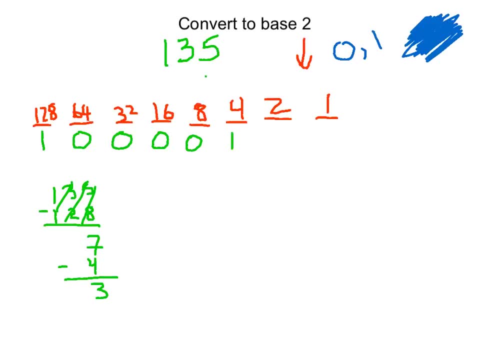 We need to make the number three using these columns here. Two goes into three one time, So we have one left over and we see that one goes in once And we got to zero. Good, So one, zero, zero, zero, zero, one, one, one.